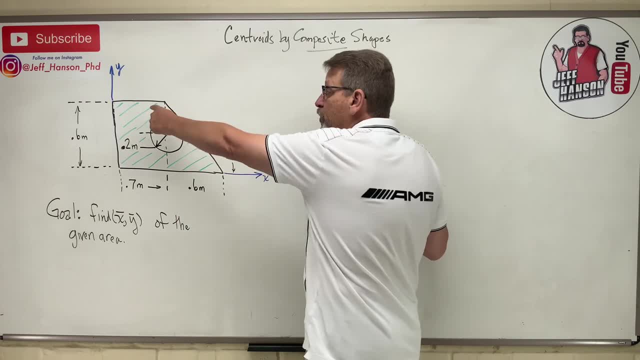 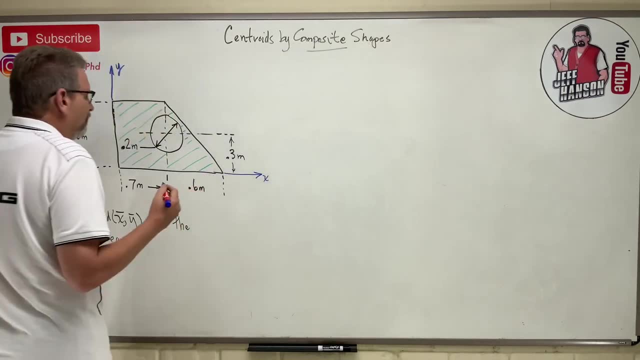 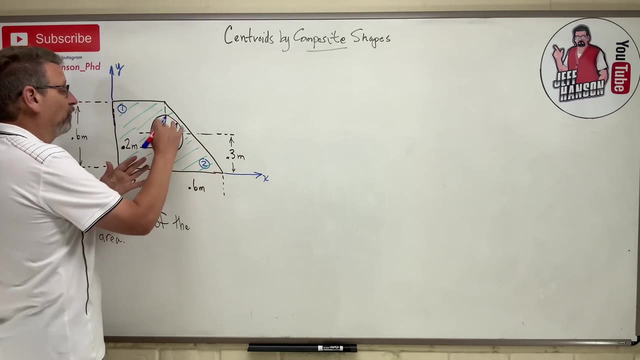 Here's our origin. over here, at this corner, You could do one big rectangle and subtract away that triangle. I don't know that that saves you anything, versus just saying, okay, I've got number one, a rectangle, number two, I've got a triangle, and number three, I'm going to subtract away that. 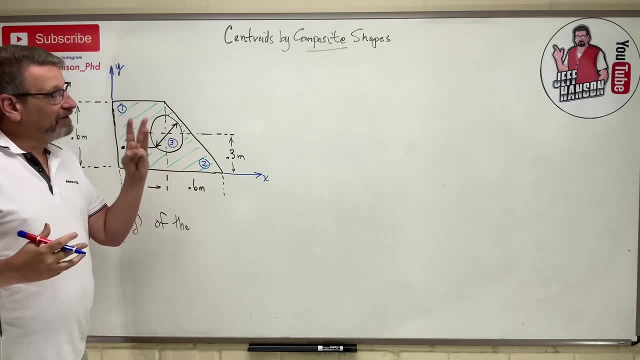 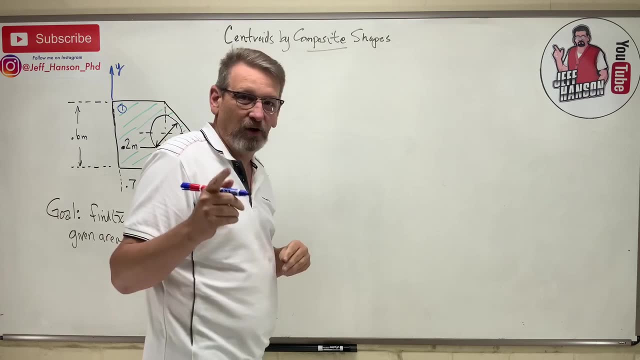 circle. okay. So three shapes. You know what? I am a fan of the table method. from now on for centroids, okay, If you're doing composite shapes, the table method is the way to go. Let's do that. So shape one, two, three. 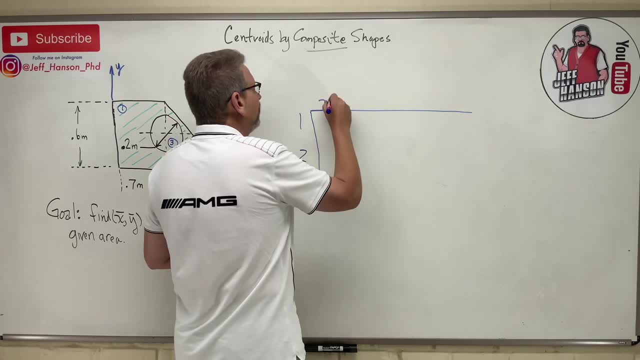 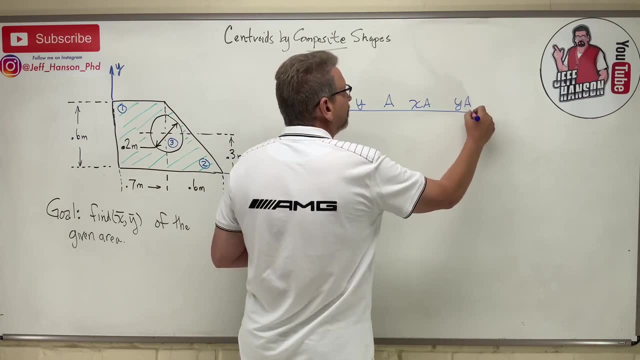 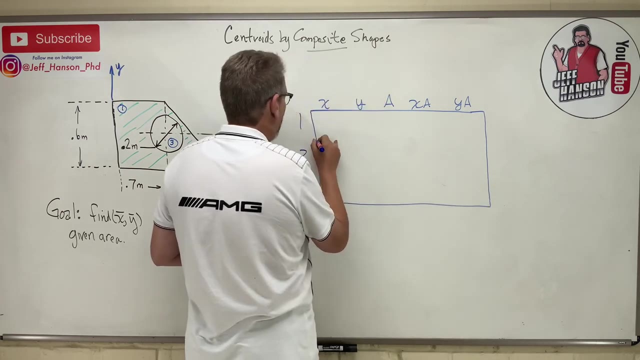 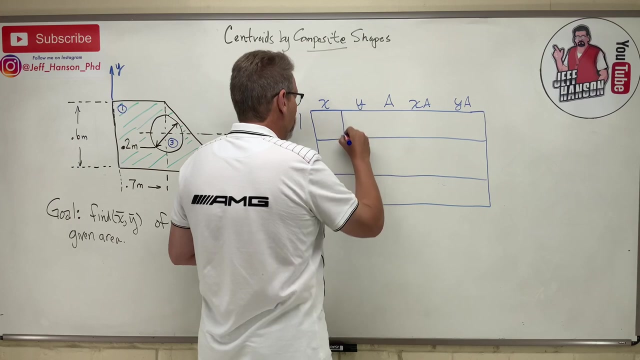 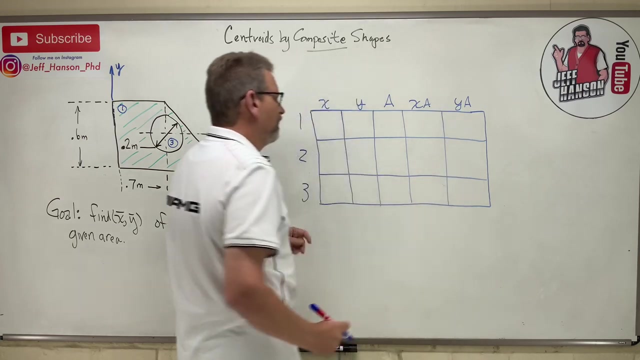 And then across the top up here I'm going to have an x-bar, a y-bar, an a, an x-a and a y-a. okay, Here we go, Okay, Okay, Making my last little table here. Look how beautiful. Remember we got to put good stuff in. 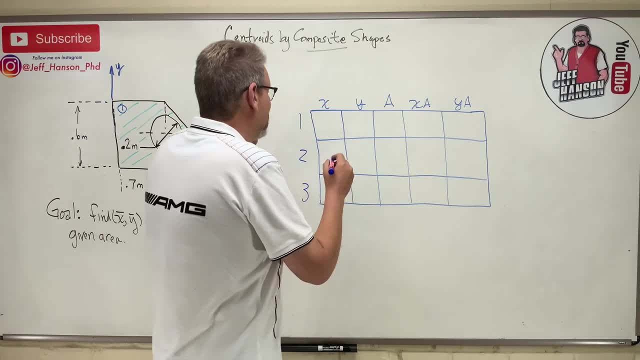 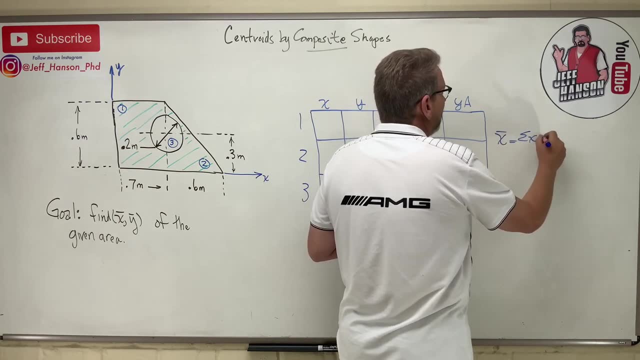 that table if we're going to get good stuff out of it And remember our centroid equation, is this? okay, I'll do it over here. X-bar is equal to the sum of the x-a's over the sum of the a's. 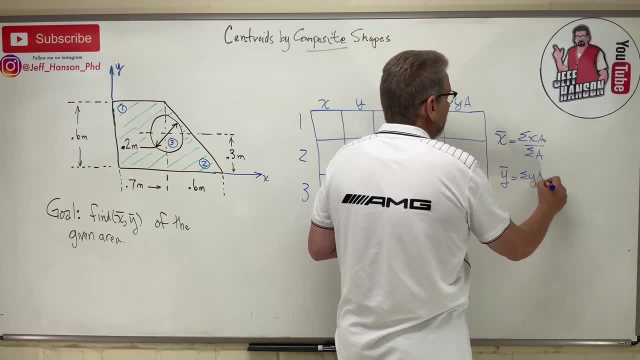 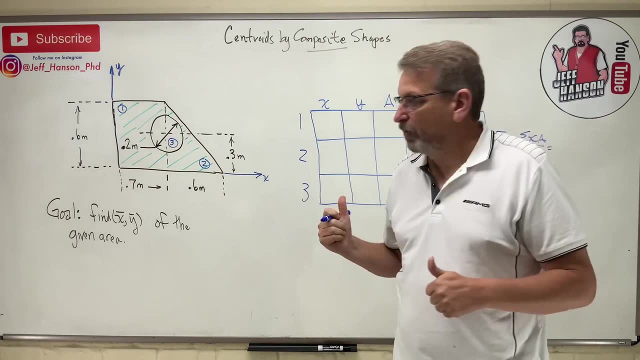 Y-bar is equal to the sum of the y-a's over the sum of the a's. So, okay, we'll get this information here from our table. Okay, so let's go. Shape number one. Shape number one: where is X bar? 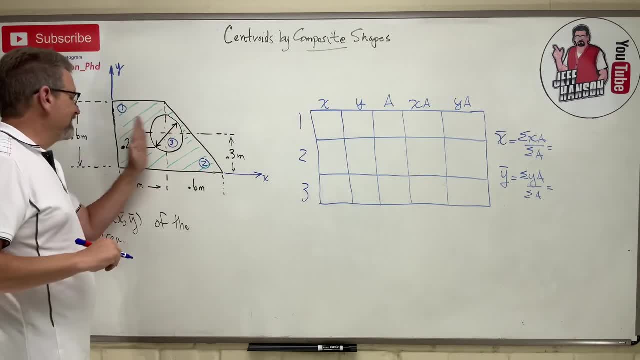 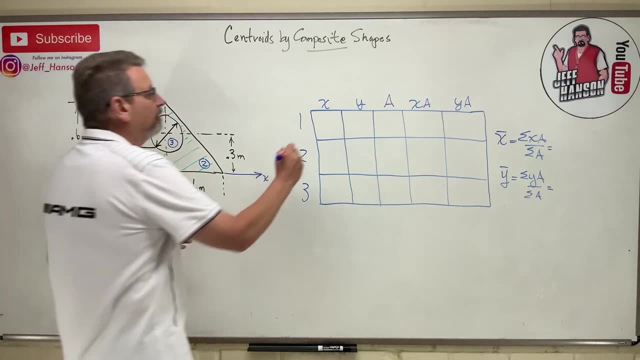 Okay, so shape number one is a rectangle. so where's half the rectangle? And just move your hand in the X direction. Okay, where in the X it's half of 0.7, which is 0.35.. And a Y bar for piece number one. 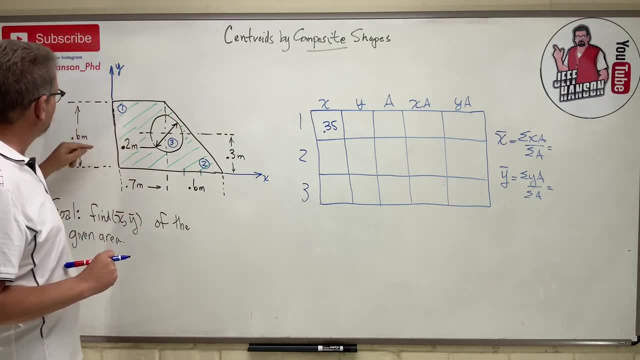 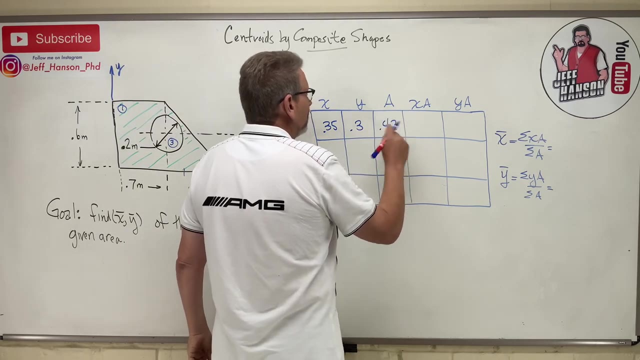 So, in the Y direction, where is piece number one? It's half of 0.6, which is 0.3.. And then the area 0.7 times 0.6, which is 0.42.. And I'll fill out the rest of that here in a minute. 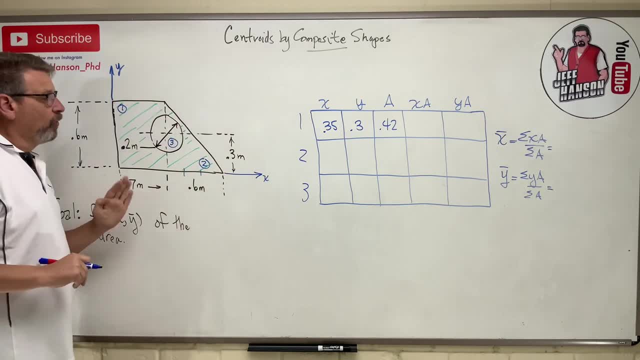 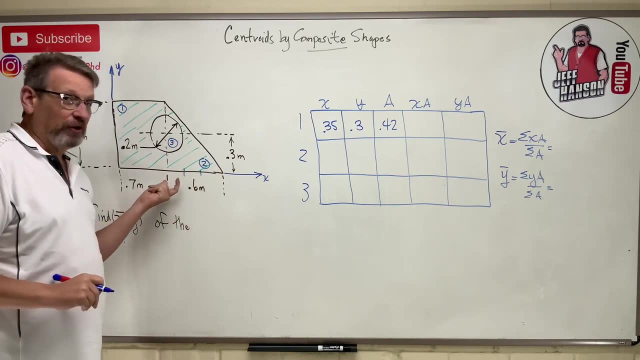 Let's go to shape number two. We're on shape number two, the triangle, Where in the X direction is the bottom of shape number two. Well, remember, for triangles, X bar for a right triangle is one third the base from the bottom of shape number two. 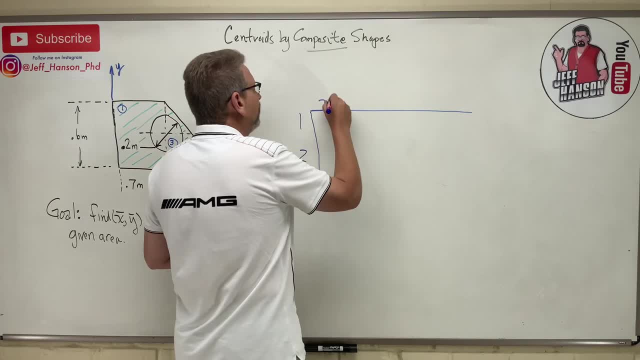 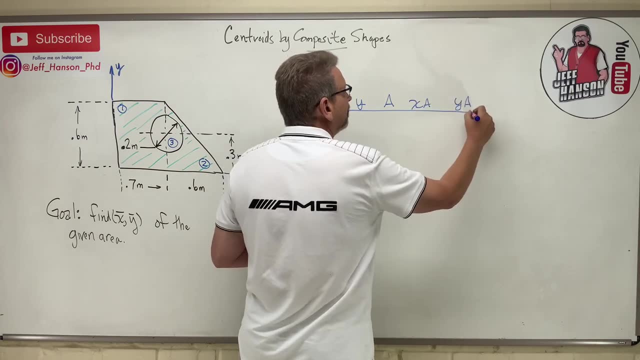 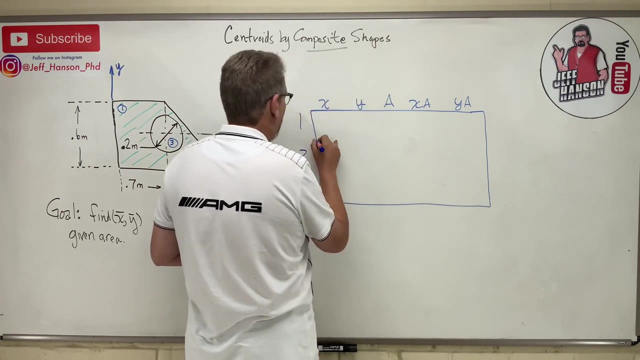 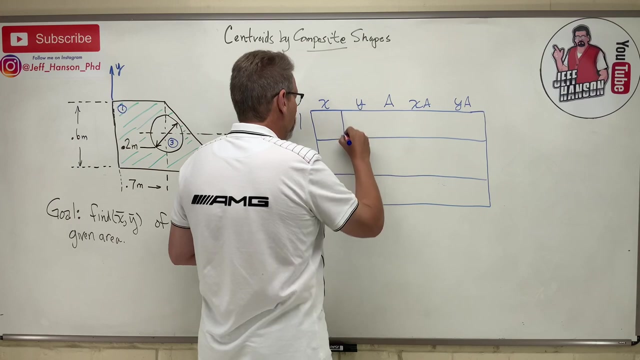 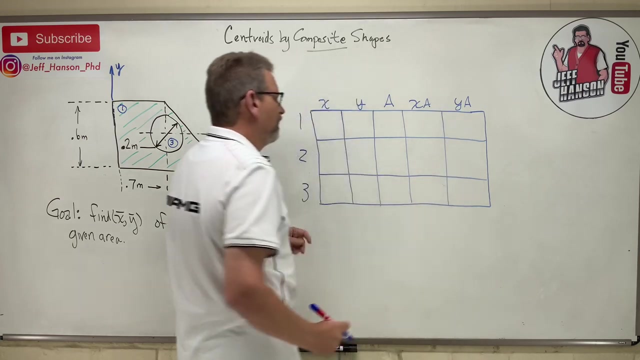 And then across the top up here, I'm going to have an x-bar, a y-bar, an a, an x-a and a y-a. okay, Here we go, Okay. Okay, I'm making my last little table here. Look how beautiful. Remember, we've got to put good. 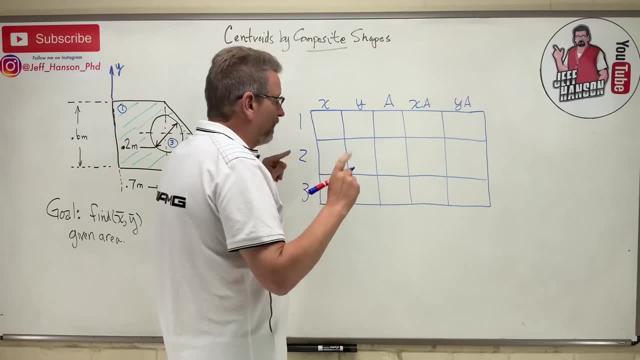 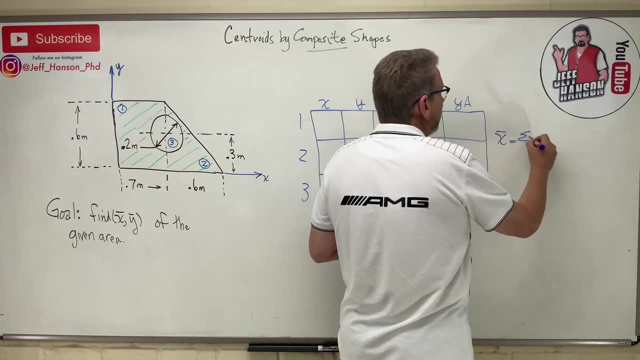 stuff in that table. if we're going to get good stuff out of it And remember our centroid equation, is this: okay, I'll do it over here. x-bar is equal to the sum of the x-a's over the sum of the a's. y-bar is equal to the sum of the y-a's over the sum of the a's. So 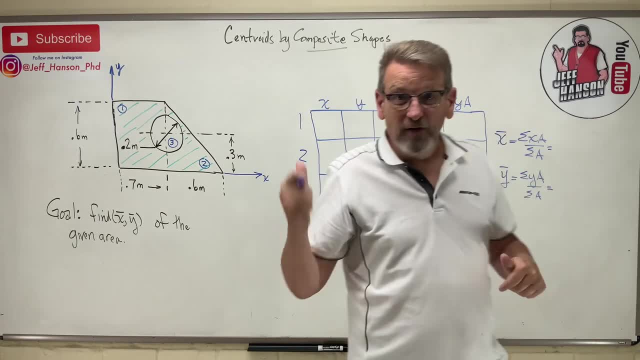 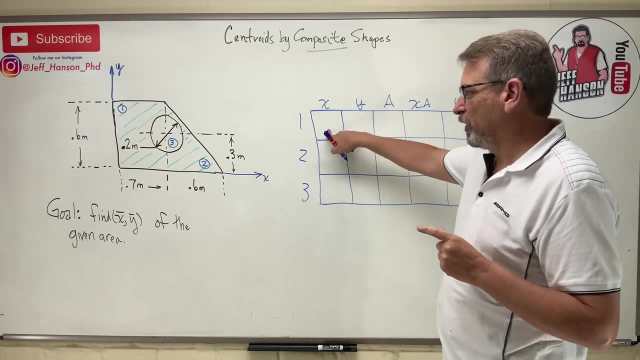 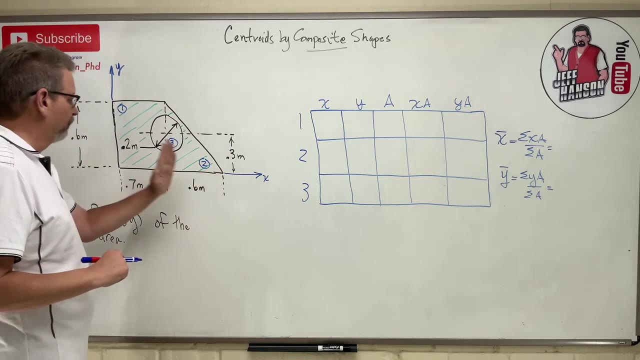 okay, this information here from our table. Okay, so let's go Shape number one. Shape number one: where is X bar? Okay, so, shape number one is a rectangle, so where's half the rectangle? And just move your hand in the X direction. Okay, where in the X It's half of 0.7, which is 0.35.. 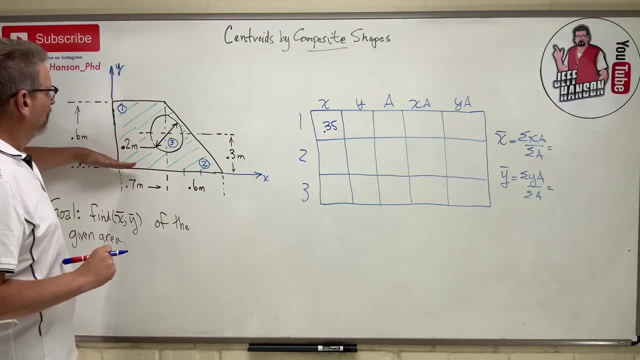 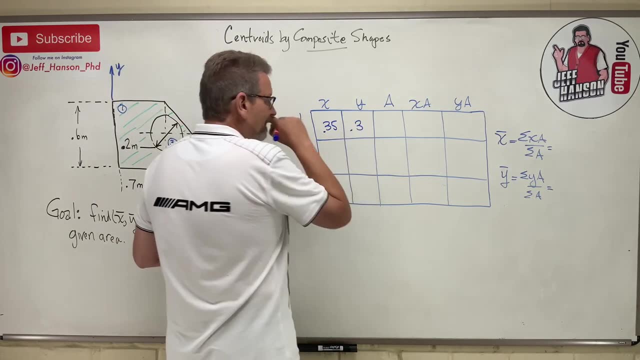 And a Y bar for piece number one. So in the Y direction, where is piece number one? It's half of 0.6, which is 0.3.. And then the area 0.7 times 0.6, which is 0.42.. 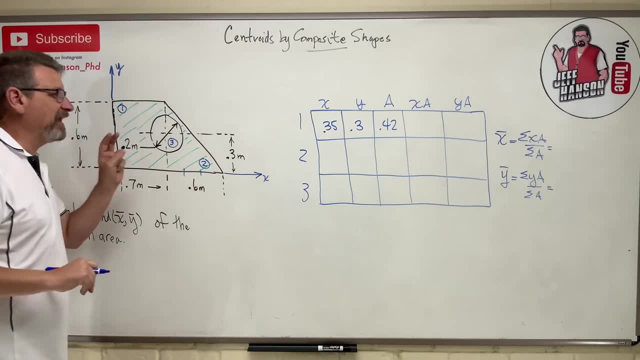 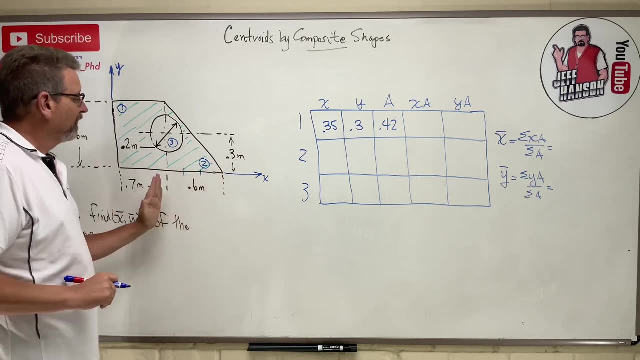 And I'll fill out the rest of that here in a minute. Let's go to shape number two. We're on shape number two, the triangle, Where in the X direction is the bottom of shape number two. Well, remember, for triangles, X bar for a right triangle is one third, the base from the fat end of the. triangle. Okay, so we're on the right side of the triangle. So we're on the right side of the triangle. Okay, so we're on the right side of the triangle. So we're on the right side of the triangle, Okay. 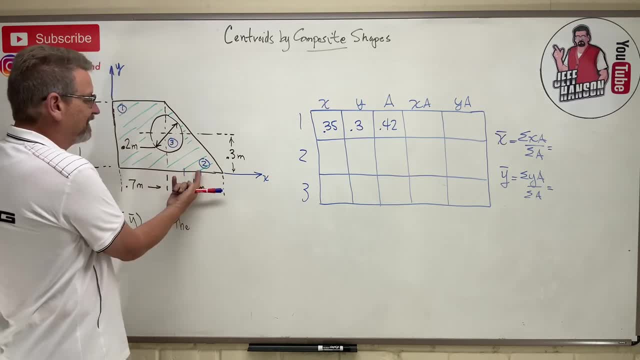 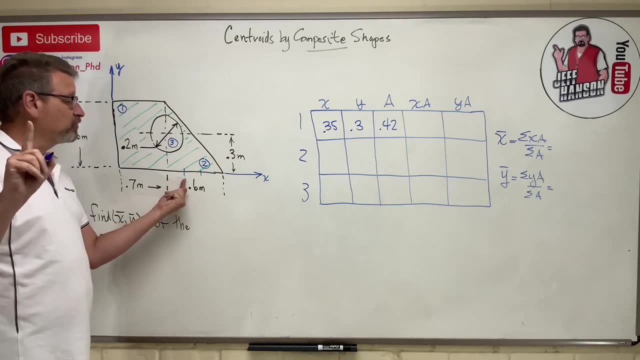 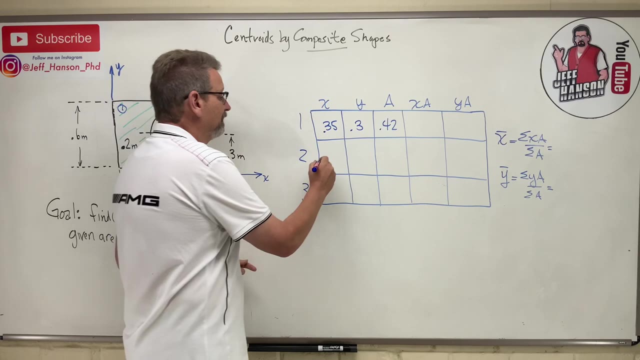 so it would be over here, Not a third from the skinny end. It doesn't make any sense that you would balance it over there. right, It's over here, So. but all dimensions are always referenced from the origin. So I got to go 0.7 to get to the triangle, then plus 0.2, which is 0.9.. Okay, 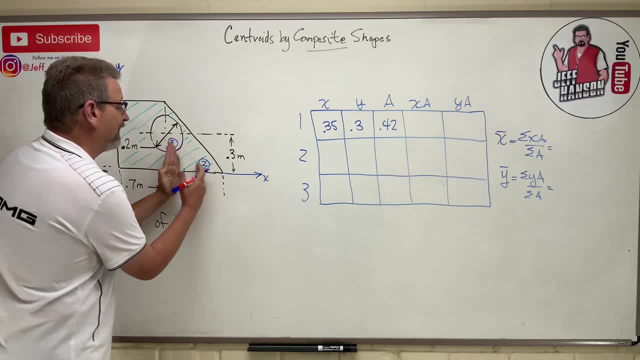 So we're on shape number two. So we're on the fat end of the triangle. okay, So it would be over here, Not a third from the skinny end. It doesn't make any sense that you would balance it over there, right? 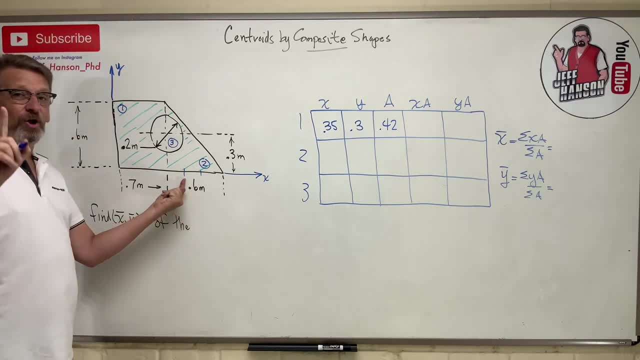 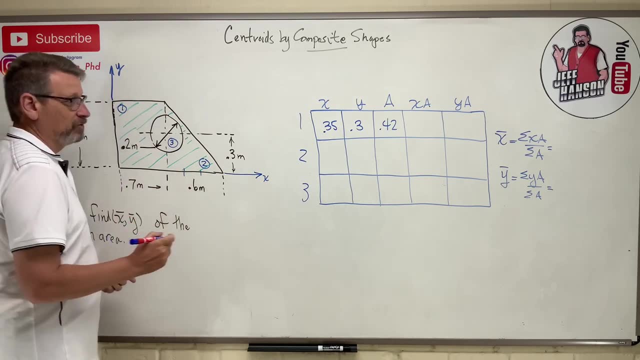 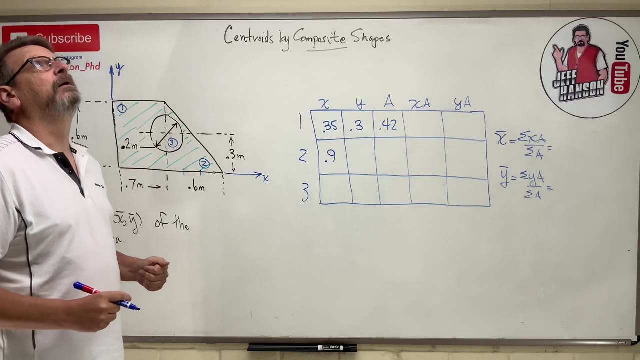 It's over here So. but all dimensions are always referenced from the origin, So I've got to go 0.7 to get to the triangle, then plus 0.2, which is 0.9.. Okay, Hey you. 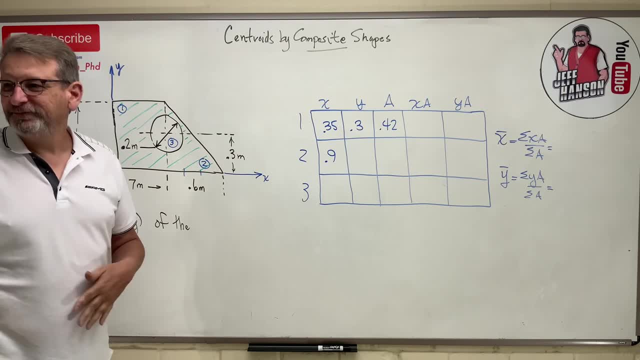 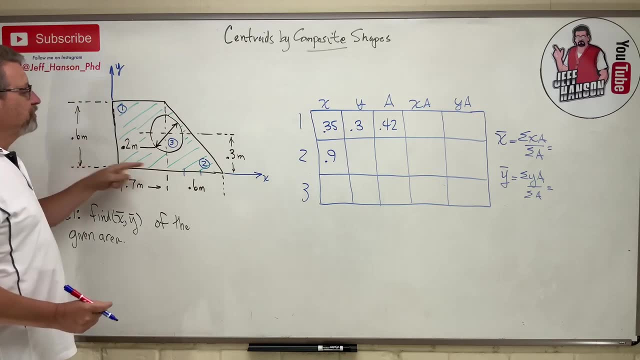 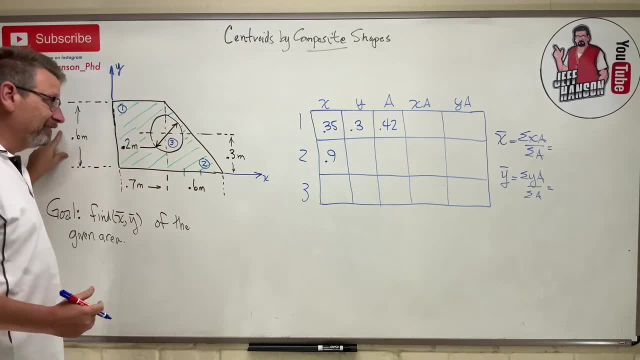 The height is a third of the height, So the height is 0.6.. So a third of that is 0.2.. And then what do we have? One half base times height. The base is 0.6.. The height is 0.6.. 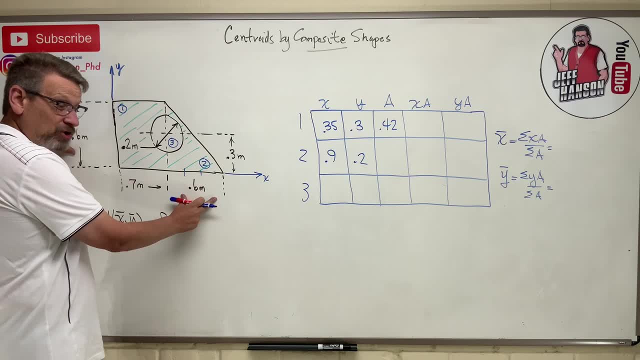 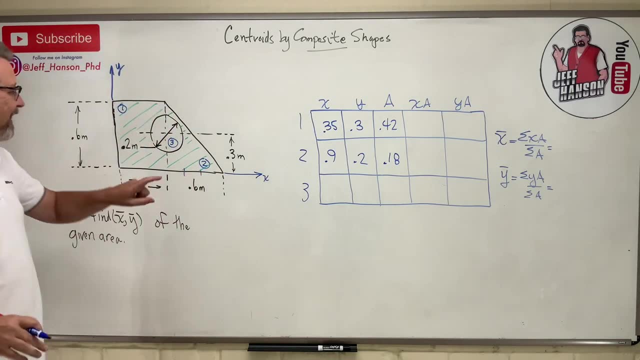 Both of them. So that's 0.2.. That's 0.3.. 0.3.. 36 divided by 2, 0.18.. Okay, we got one more to go, and that is shape number 3, okay. 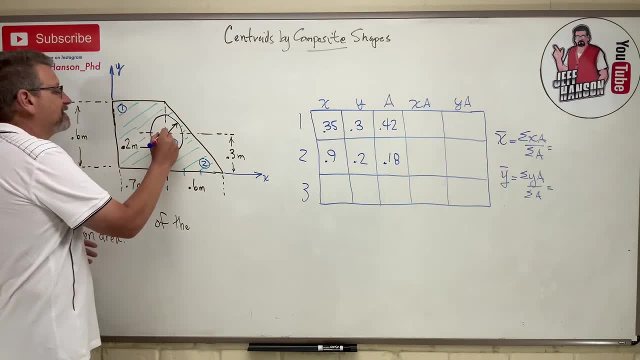 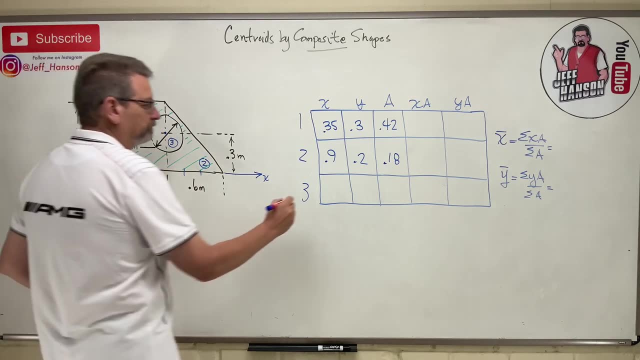 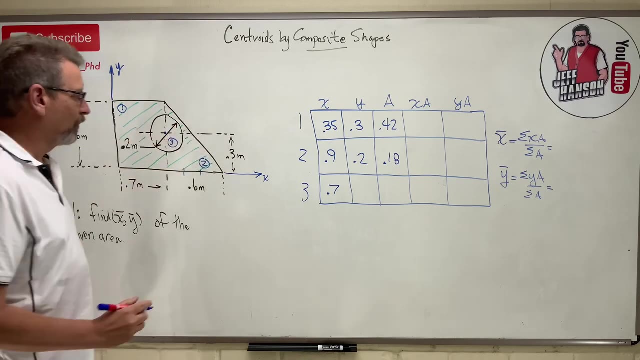 So where is X-bar for shape number 3?? Well, shape number 3, it's centrally, it's like right in the middle of the circle. So X-bar is at whoop bam 0.7.. Okay, and Y-bar? where is it Y-bar? well, it's whoop 0.3.. 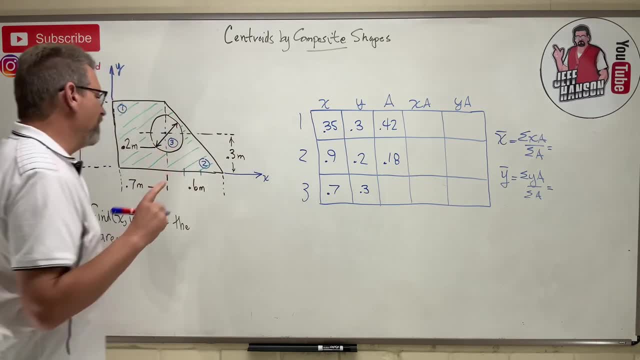 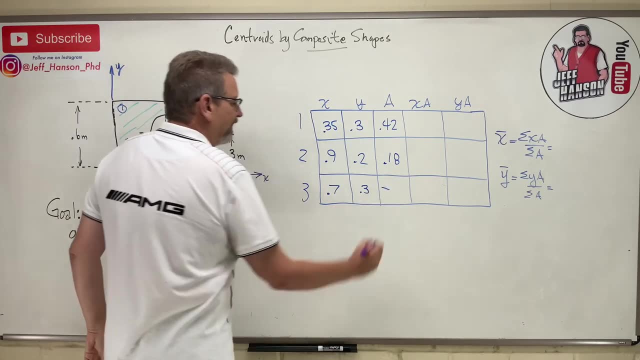 Okay, and the area? this is the tricky part. not really that tricky. the area is not really there. so I know for a fact the area is going to be a negative. okay, got to be. And what is the area? 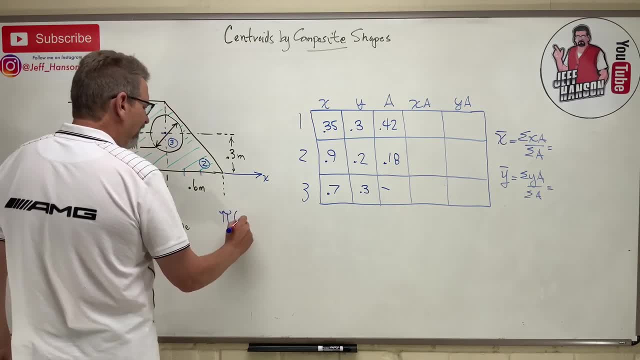 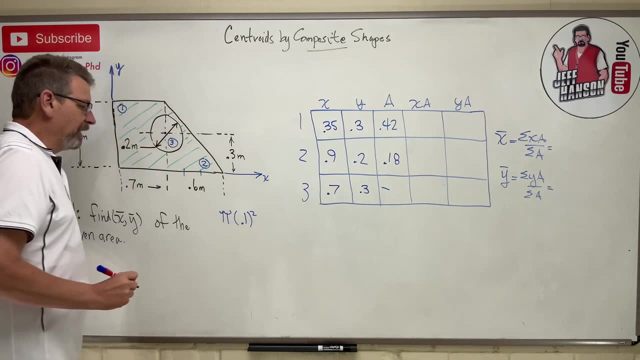 It's just pi or squared, isn't it Pi times they gave me? the diameter is 0.2, so that's 0.1 squared. okay, and that is duh. that's probably easy. you all got it already, right. 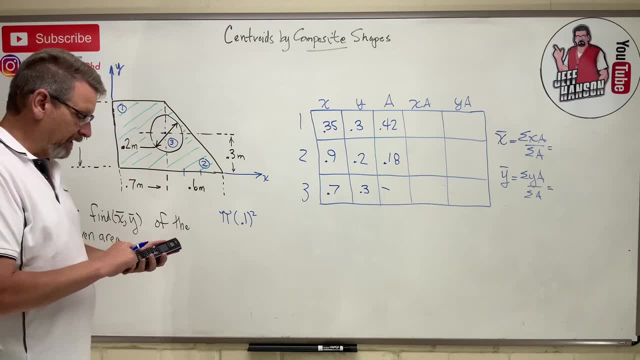 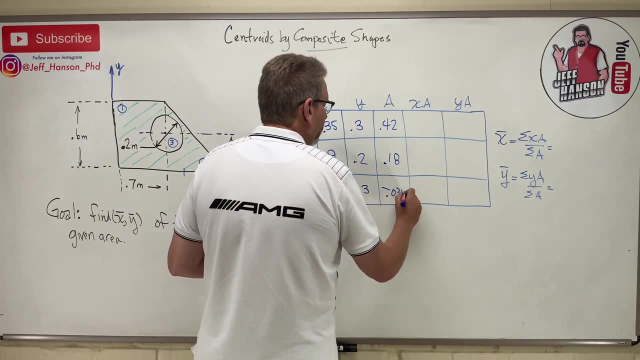 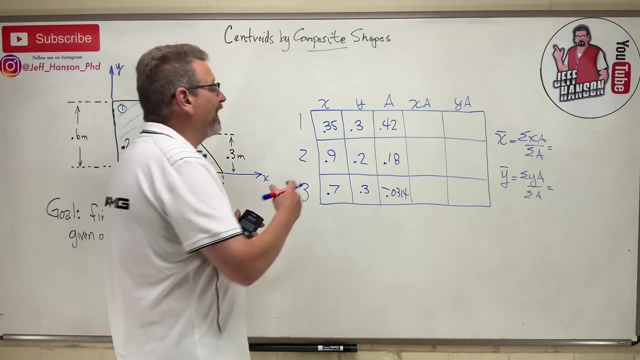 Uh, 0.1 squared times pi equals 0.0314,, 0.0314, okay, and those are in meters, so this is a. that's a little number there, isn't it? So now all we have to do is just multiply the rest of our table out, so 0.35 times 0.42. 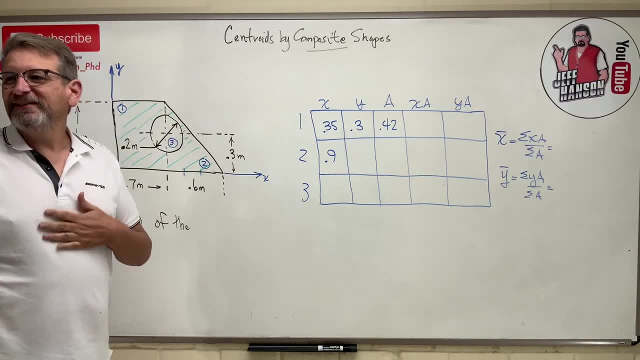 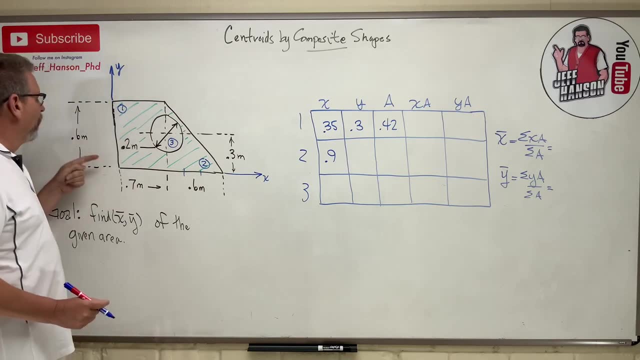 Hey, you Give me. So what is Y bar for shape two? Here's shape two. What is Y bar? Okay, Right, triangles, Like the base is a third of the base, The height is a third of the height, So the height is 0.6.. So a third of. 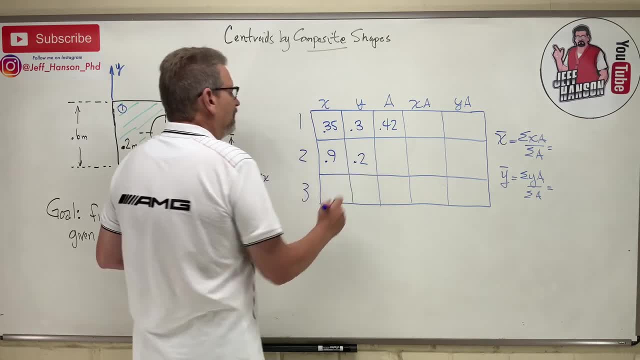 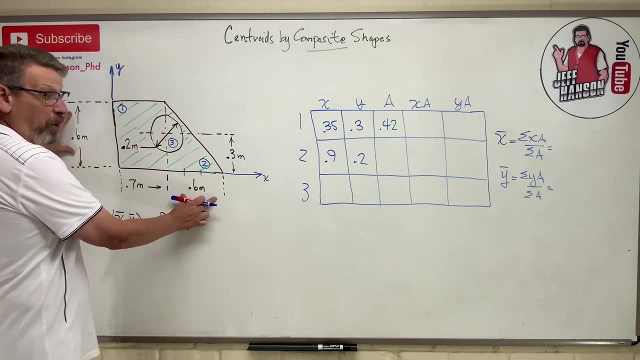 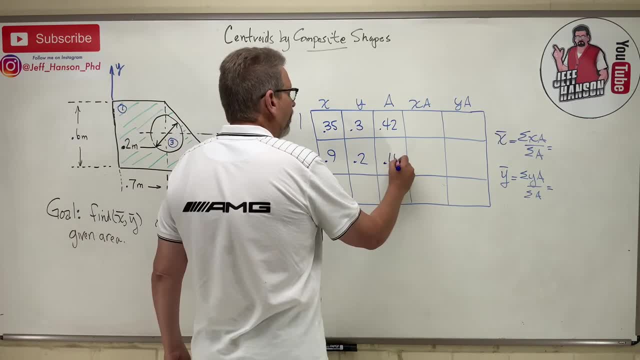 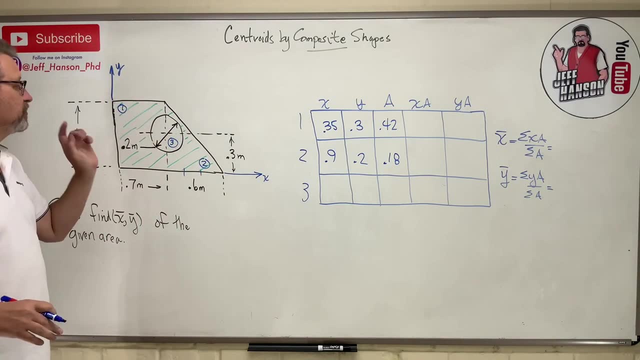 divided by two, 0.18.. Okay, We got one more to go, and that is shape number three. Okay, So where is X bar for shape number three? Well, shape number three is it's centrally, it's like right. 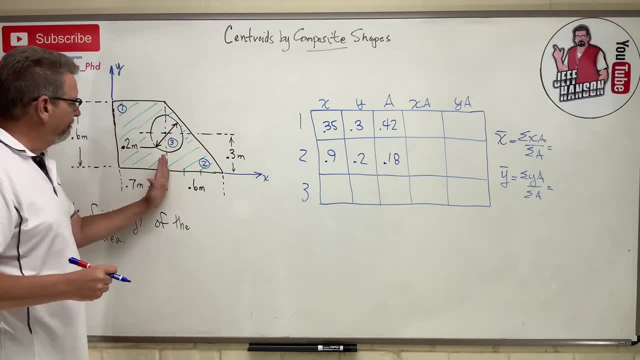 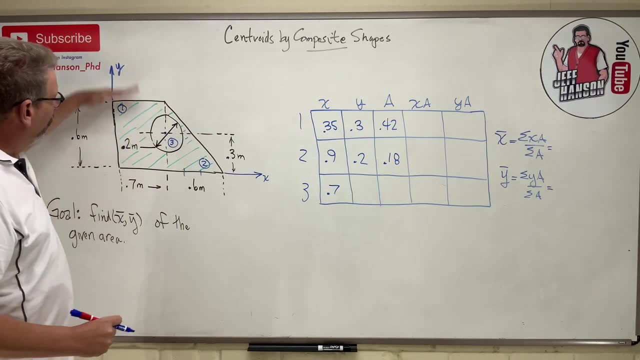 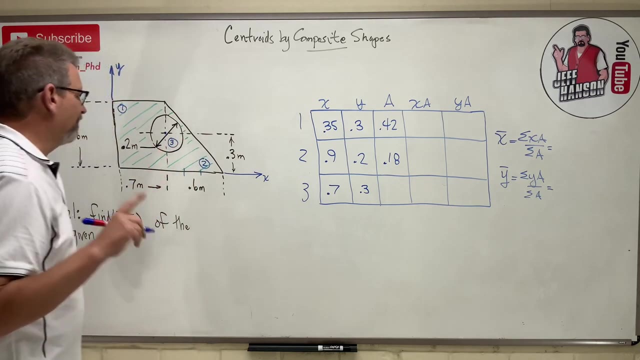 in the middle of the circle. So X bar is at 0.7.. Okay, And Y bar. where is it? Y bar? Well, it's 0.3.. And the area. this is the tricky part. Not really that tricky, The area is not really there. So I 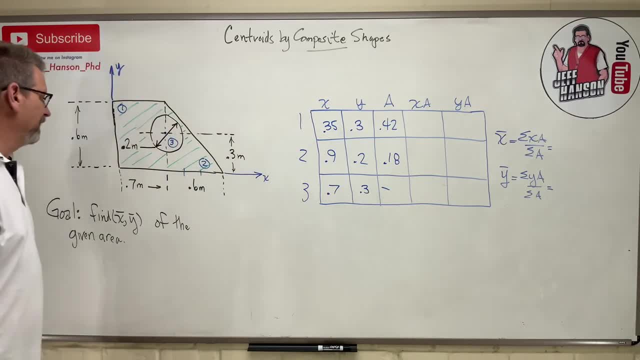 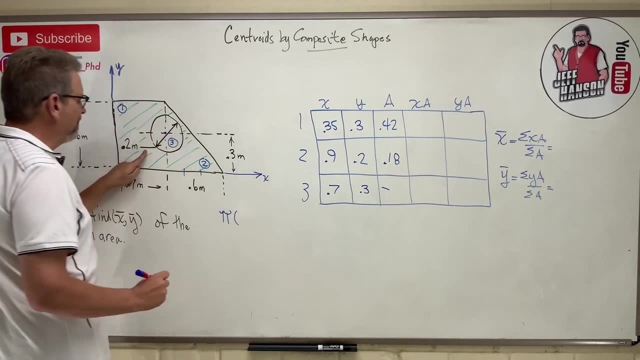 know for a fact: the area is going to be a negative. Okay, Got to be. And what is the area? It's just pi squared, isn't it? Pi times? they gave me the diameter is 0.2.. So that's 0.1 squared, Okay, And 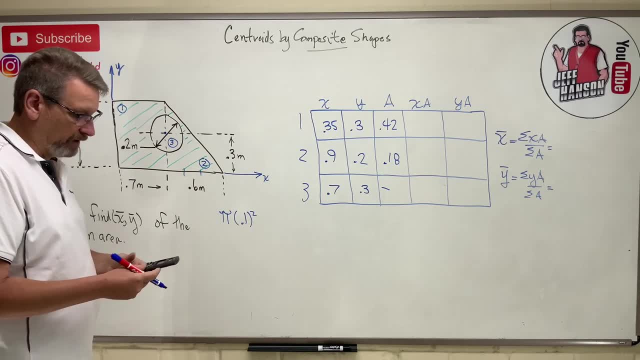 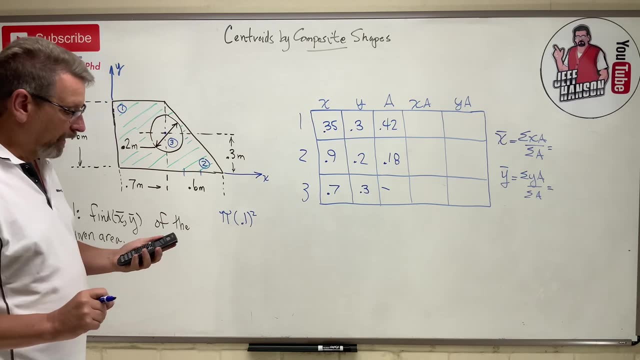 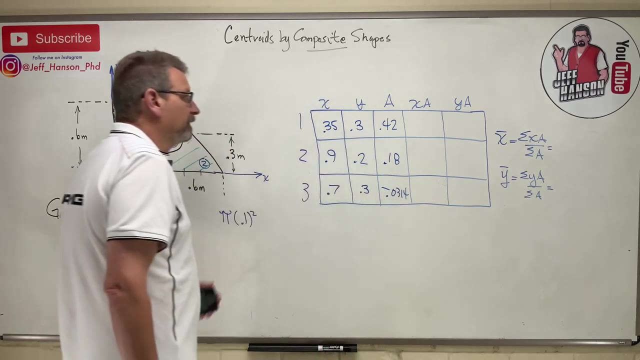 that is duh. That's probably easy And y'all got it already right: 0.1.. 0.1 squared times pi equals 0.0314.. 0.0314.. Okay, And those are in meters, So this is a. 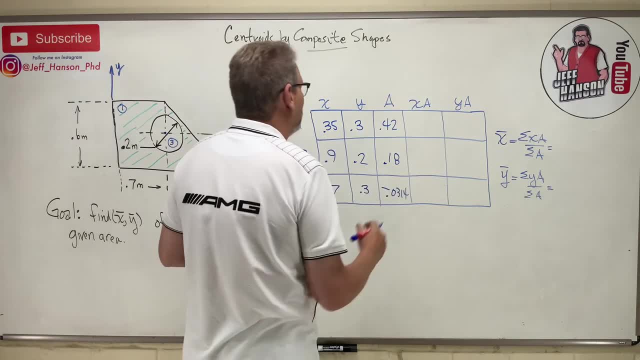 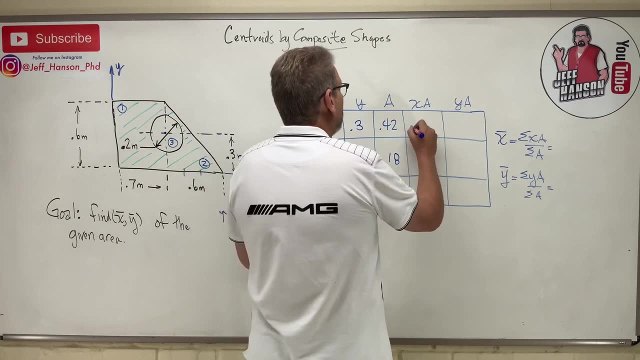 that's a little number there, isn't it? So now all we have to do is just multiply the rest of our table out. So 0.35 times 0.42 equals that's 0.147.. And then 0.3 times. 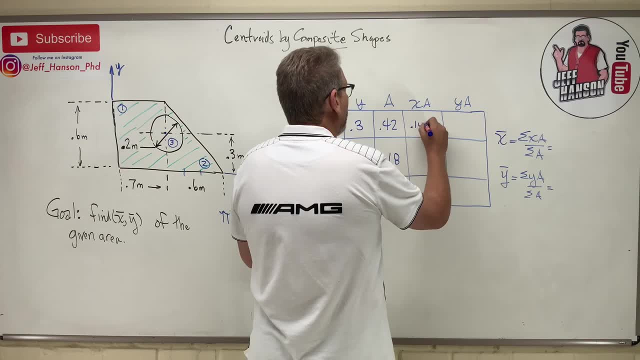 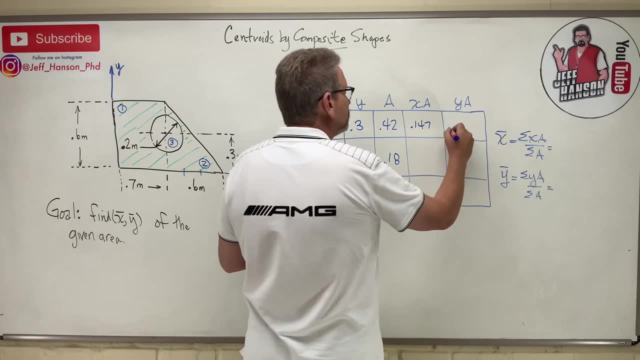 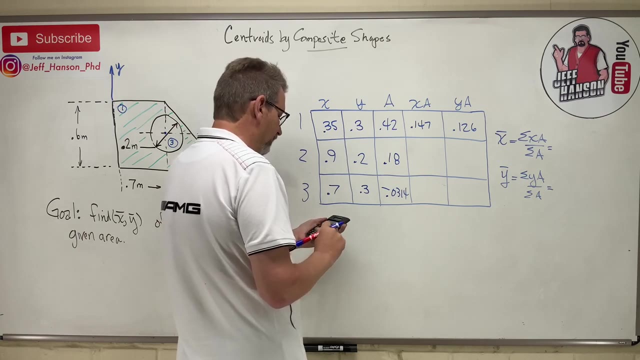 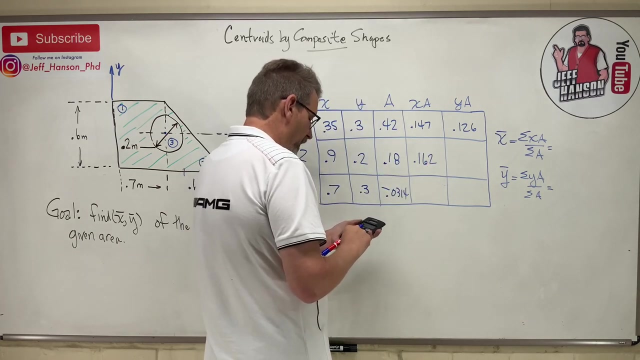 equals, that's 0.147.. And then 0.3.. Times 0.42,, that's 0.126,, and then 0.9 times 0.18 is 0.162,, and then 0.2 times 0.18 is. 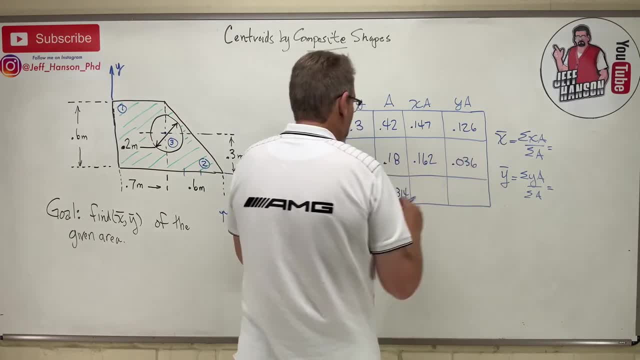 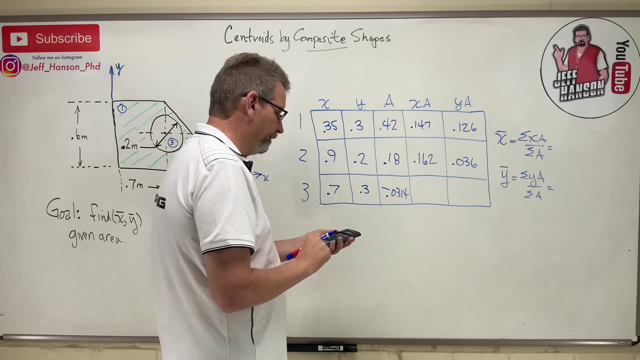 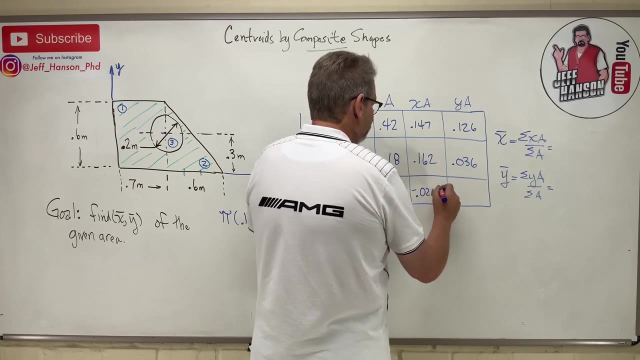 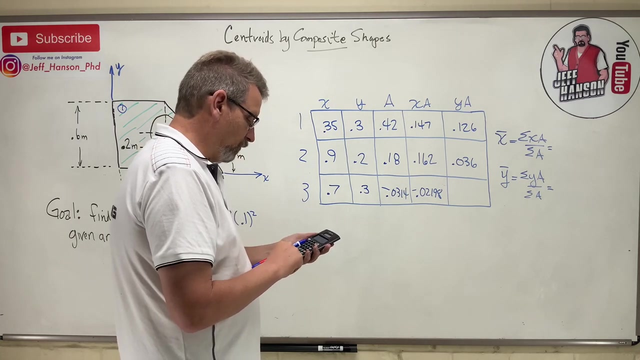 0.036,, and then finally 0.7 times negative: 0.0314 is 0.036,, and then 0.2 times 0.18 is point negative: 0.02198,. and then one more 0.3 times negative: 0.0314 equals negative. 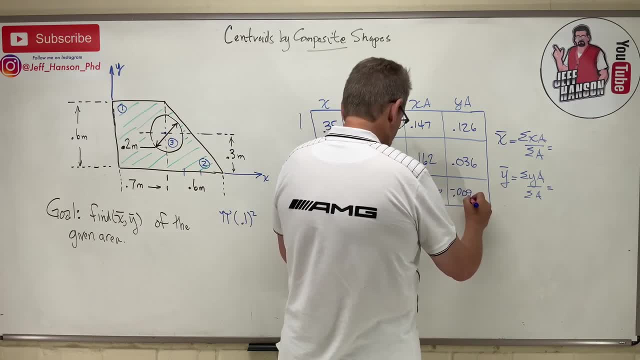 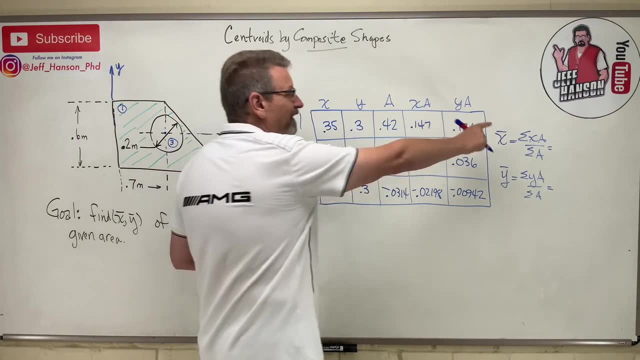 0.00942,. okay, All right. so what we need over there is: we need the sum of the x's, and we need the sum of the a's and we need the sum of the y's, Don't we? Well, where are we going to get that? 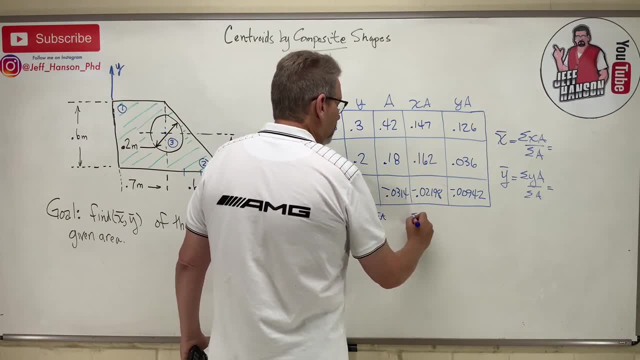 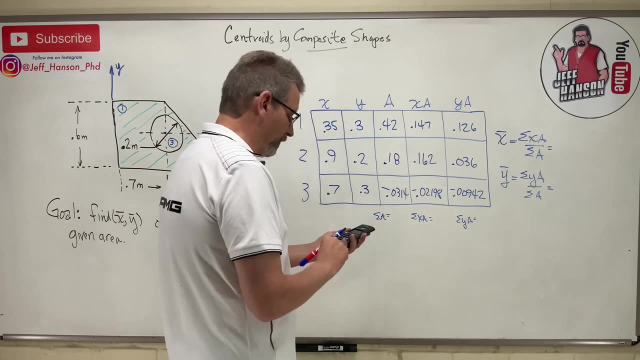 Well, that's easy. Sum of the a's comes from this column, sum of the x's come from that column and the sum of the y's come from that column. okay, All we got to do is add this stuff up. so here we go: 0.42 plus 0.18 minus 0.0314 equals. 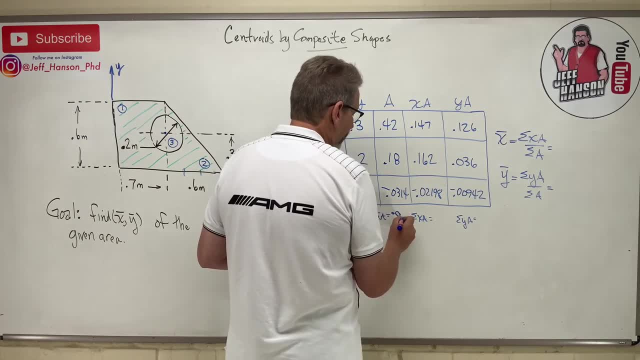 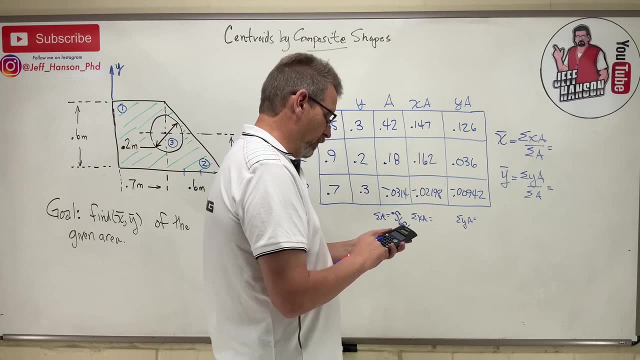 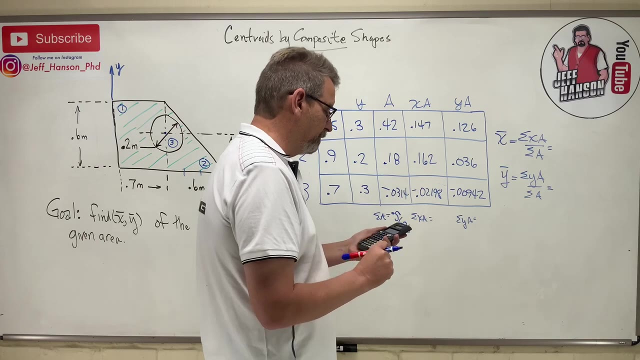 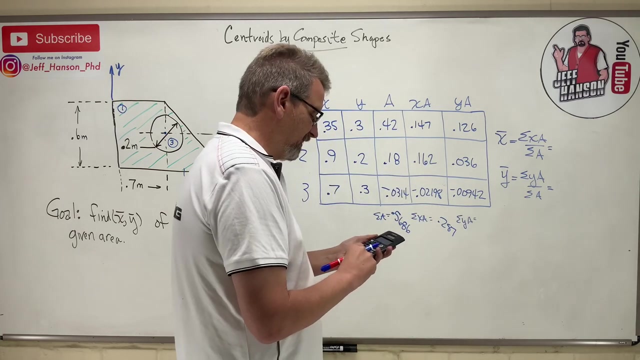 0.5686,. okay, The sum of the x's 0.147. Plus 0.162 minus 0.02198 is 0.287, and then the sum of the y's 0.126 plus 0.036 minus. 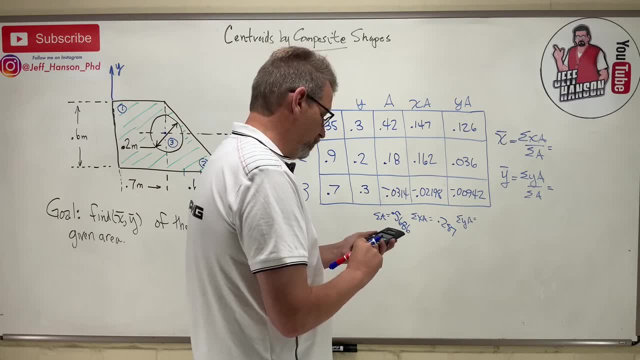 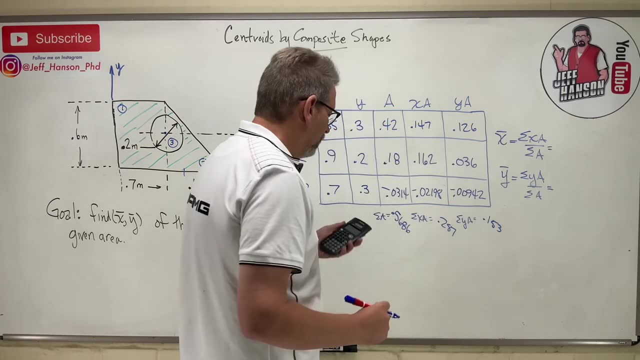 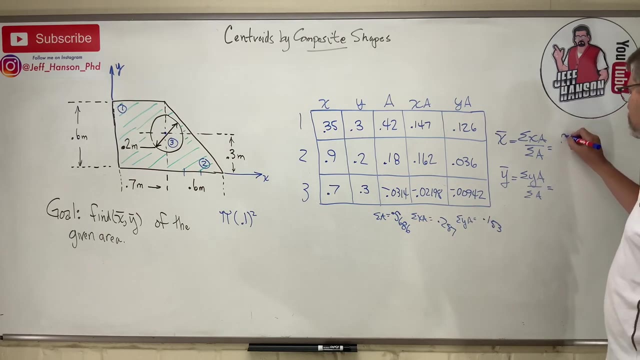 0.00942 is 0.153,. okay, And so here we go: x bar. x bar is the sum of the x's 0.287 divided by 0.5686, and then y bar is going to be 0.153 divided by 0.5686, okay. 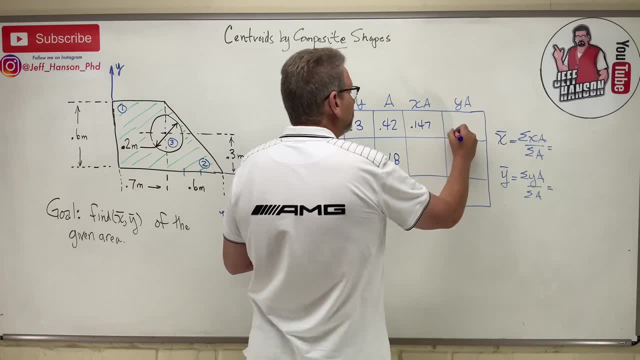 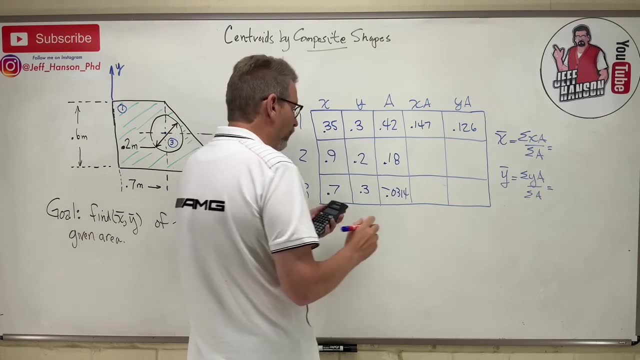 0.2 equals 0.126.. 0.5 times 0.0615.. And then 0.9 times 0.18, is 0.162.. 0.2 times 0.18 equals 0.036.. 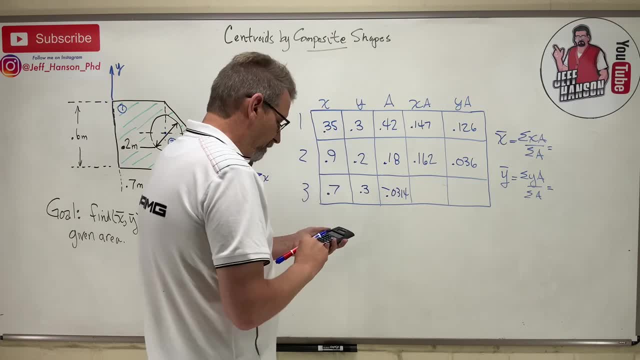 0.3 times 0.18 equals 0.046.. And then 0.7 times negative: 0.0314, equals 0.036.. 0.3 times 0.018 equals 0.0316.. 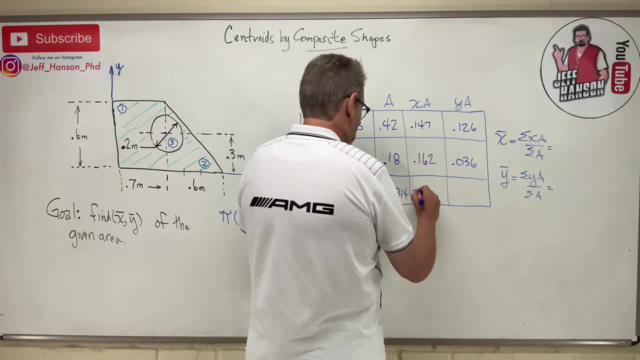 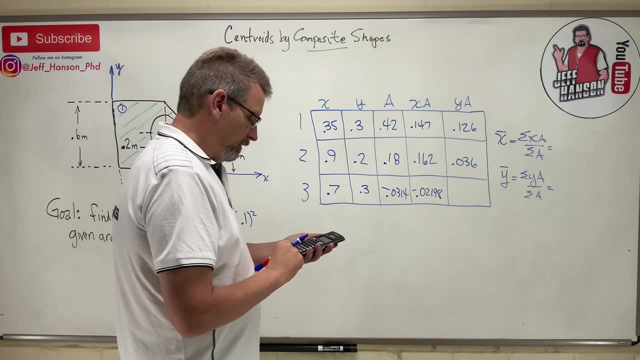 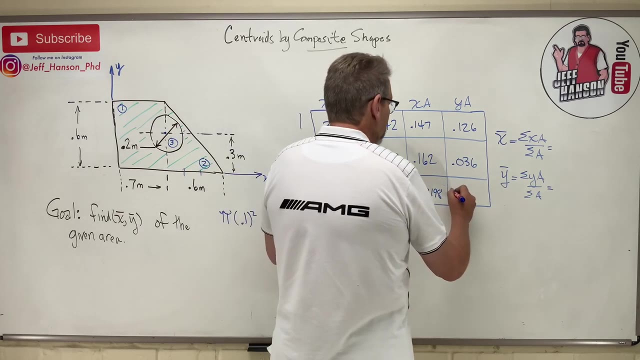 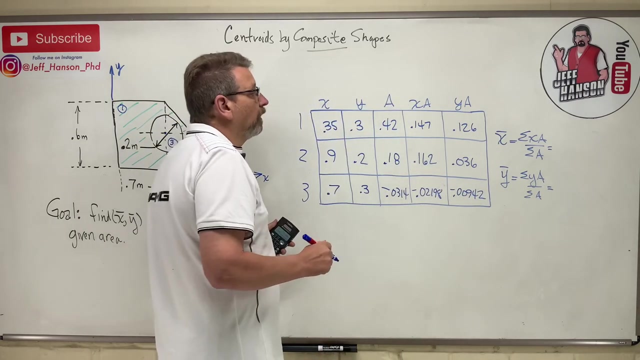 0.2 times 0.018 equals 0.036.. is point negative point zero: two, one, ninety, eight. and then one more point, three times negative point: oh, three, one, four equals negative point zero. zero, nine, four, two. okay, all right, so what we need over there? 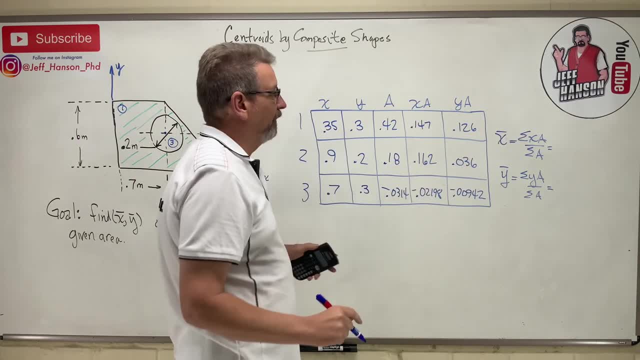 is: we need the sum of the x a's, and we need the sum of the a's, and we need the sum of the y a's, don't we? well, where are we going to get that? well, that's easy. some of the a's comes from this column. 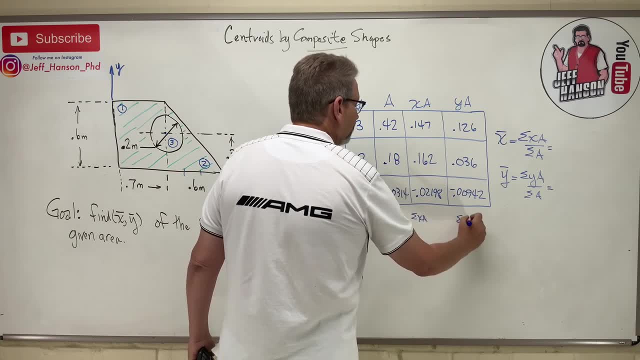 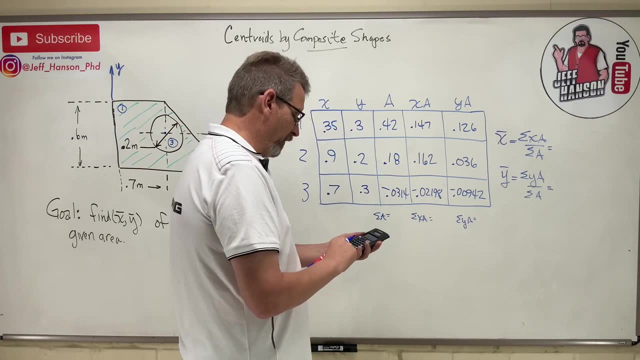 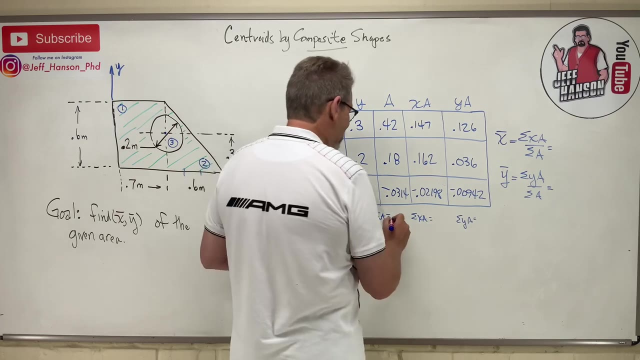 some of the xa's come from that column and the sum of the y a's come from that column. okay, all we gotta do is add this stuff up. so here we go. 0.42 plus 0.18 minus 0.0314 equals 0.5686. 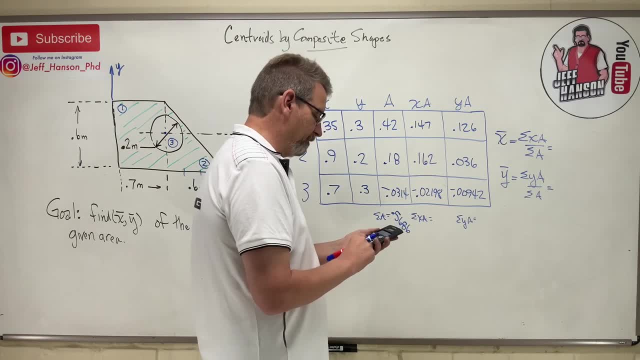 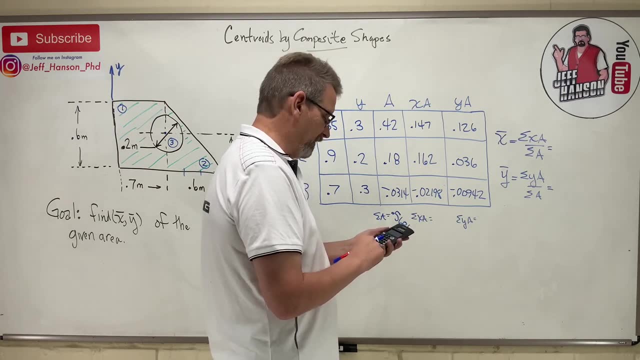 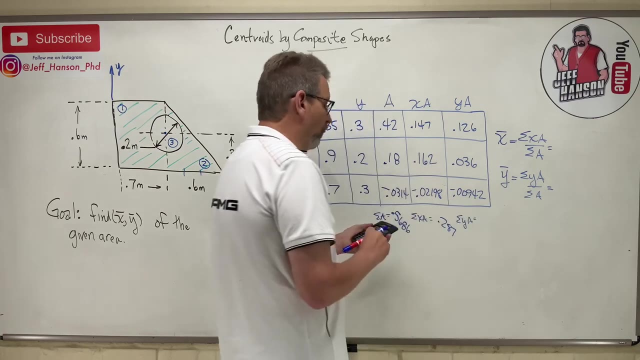 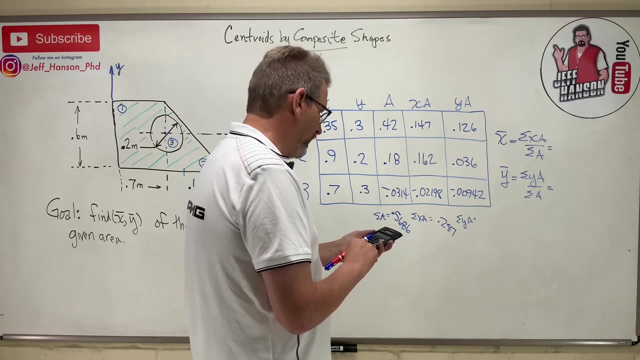 okay, the sum of the xa's 0.147 plus 0.162 minus 0.02198 is 0.287, and then the sum of the y a's 0.126 plus 0.036 minus 0.00942 is 0.153. 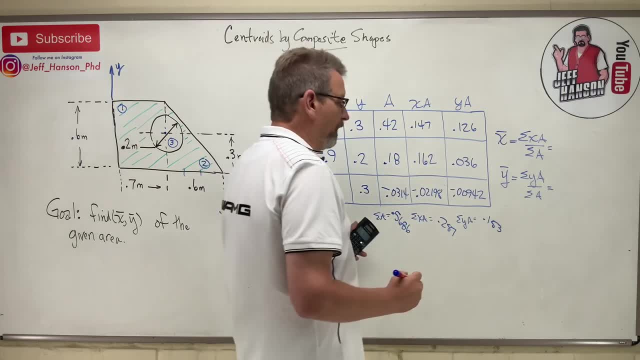 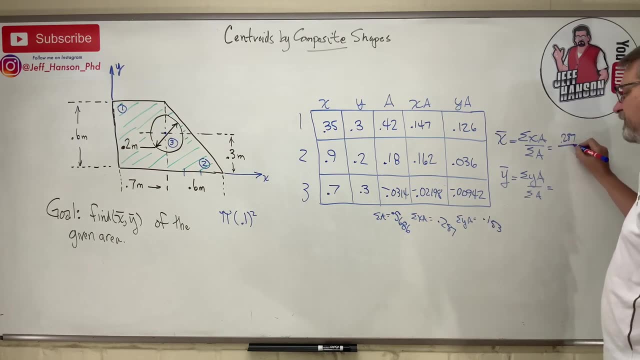 okay, and so here we go: x bar. x bar is the sum of the x a's 0.287 divided by 0.5686. and then y bar is going to be 0.153 divided by 0.5686. okay, we're one calculator away: 0.287 divided. 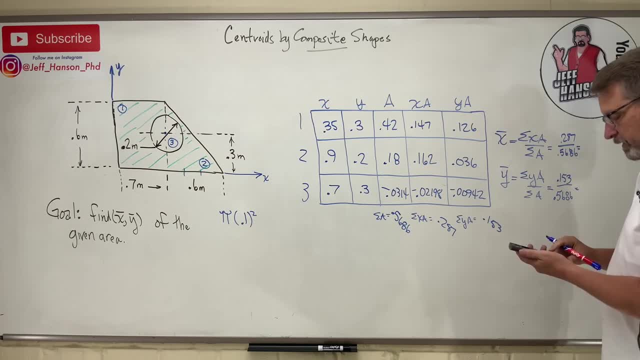 We're one calculator away: 0.287 divided by 0.5686.. Equals 0.505, and these were in meters, weren't they? There's x bar, and then 0.153 divided by 0.5686, 0.269, and there is y bar. okay. 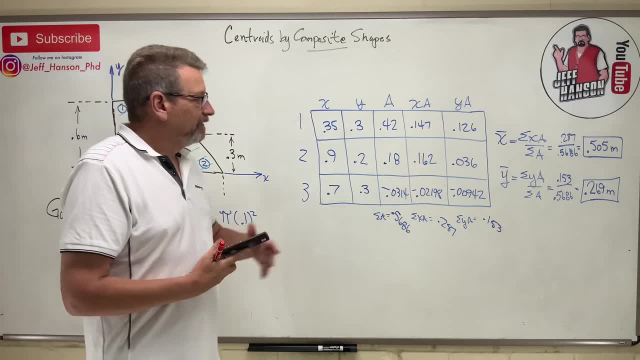 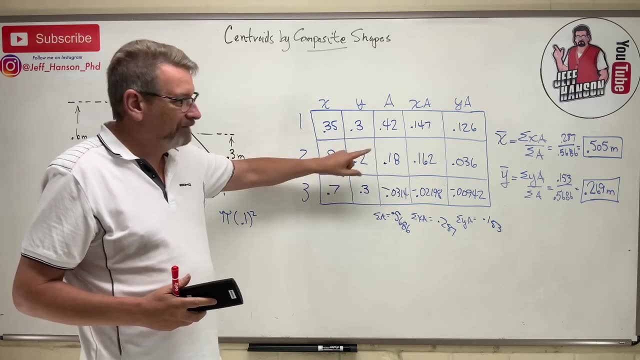 So I think these are really nice. When you just make these little tables, you've got to be super careful about every single little thing you put in your table, because one mistake and then your answer's wrong. So hope that helps. That's the method of composite shapes. See you next time. 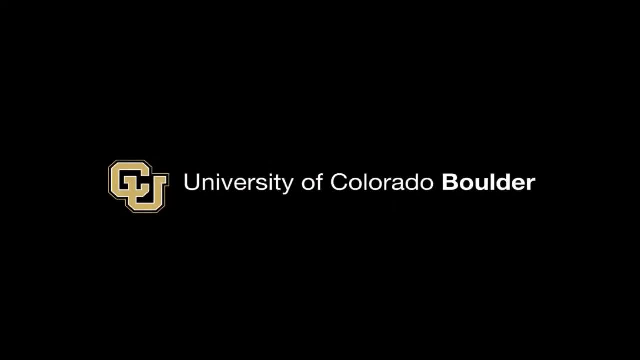 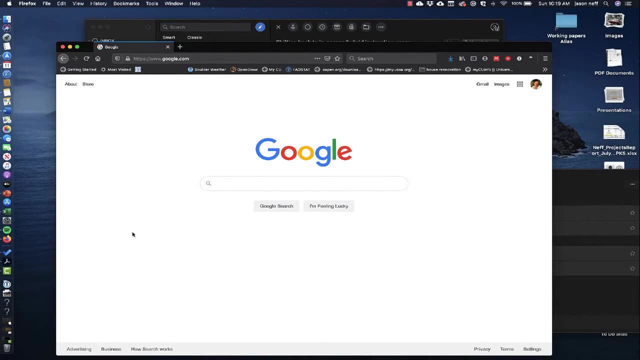 In this video I'm going to show you how to navigate to the FAO data that we're going to use to look at agricultural yields. Now, this data is in a database called FAO Stat, and the easiest way to find it is actually just to type that into Google or another search. 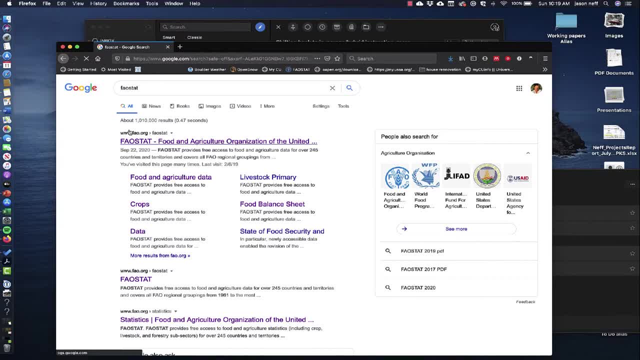 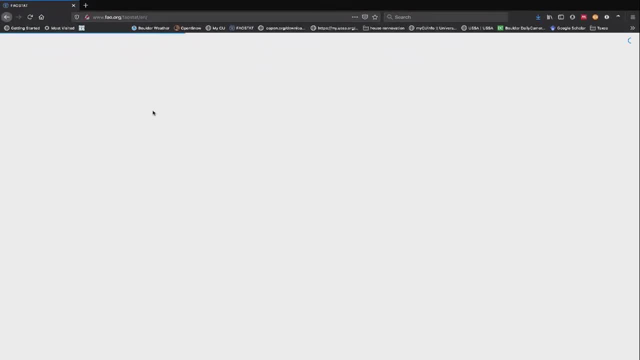 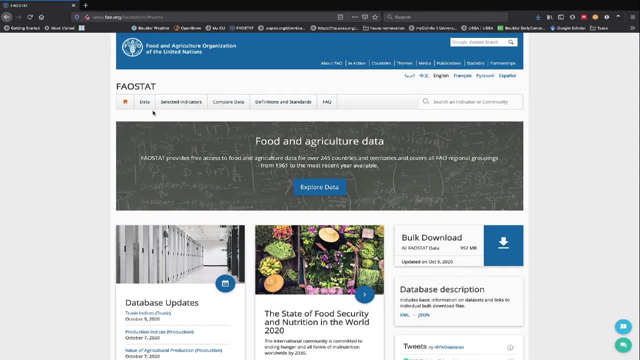 engine and usually your first hit will be this FAO Stat. It's from faoorg Click that The Food and Agriculture Organization is run out of the United Nations. They collect data on agricultural statistics. They do some really interesting reports on agricultural trend. 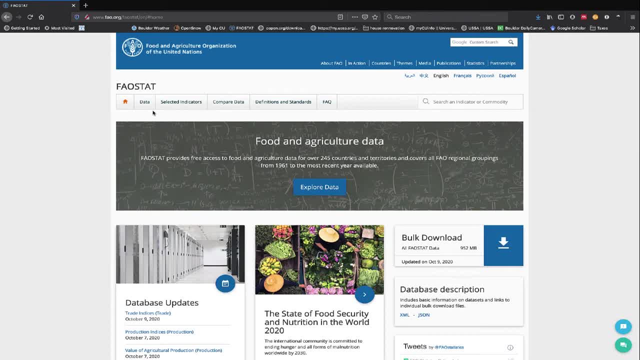 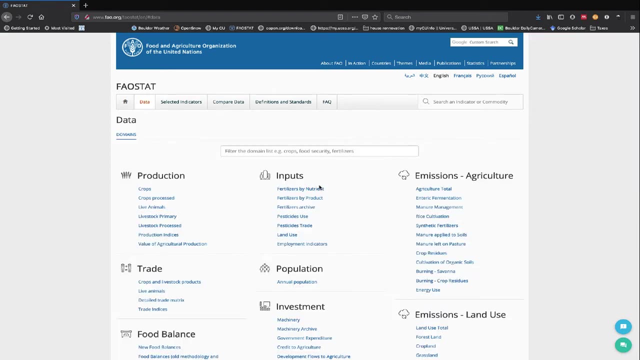 and the data access is actually one of the better sources of data that you can find. So this is actually a pretty neat site for a lot of different things. Two ways in. You can go in via data up on the upper left hand corner, or you can just explore data and you'll get to a page like: 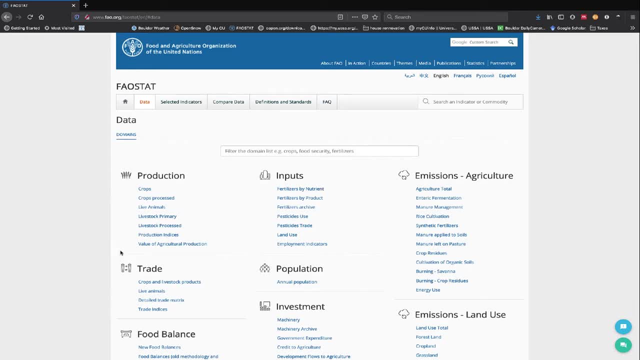 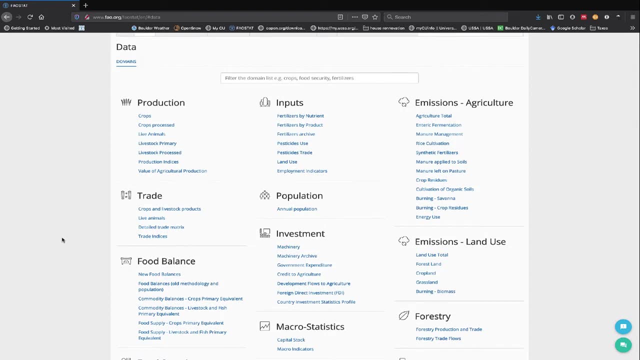 this FAO Stat tracks a lot of different things. You can see production trade, food balances if you're interested in malnutrition, food balances, the statistic block that you would want to use For us, though. we're interested in crops and we're interested in production.